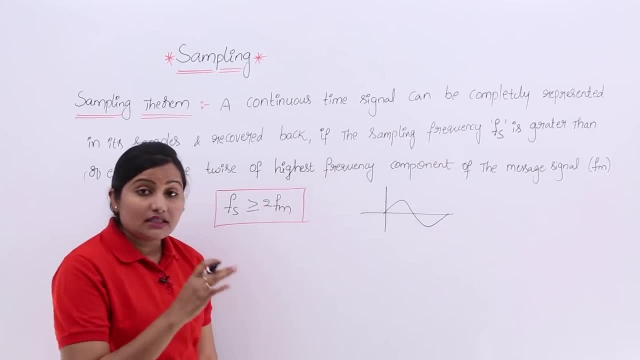 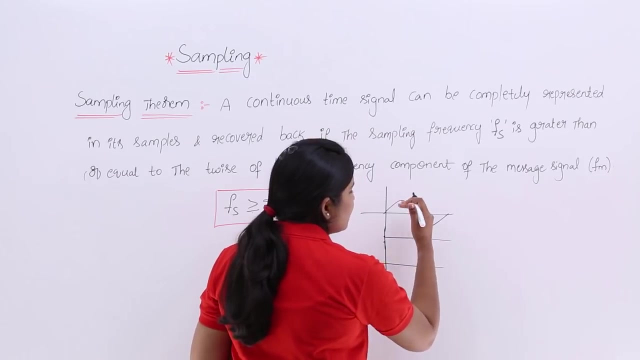 time signal like this. I am considering a sign signal. This signal we can completely represent into its samples. So we can completely represent into its samples by multiplying the number of samples multiplied by the frequency fs. How we can convert, how we can completely convert this signal into its samples, means just by multiplying a pulse. trying with the 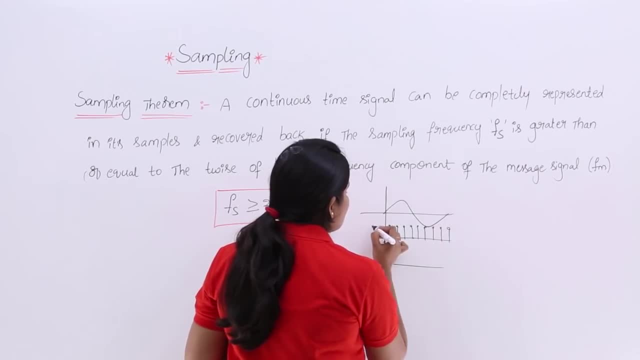 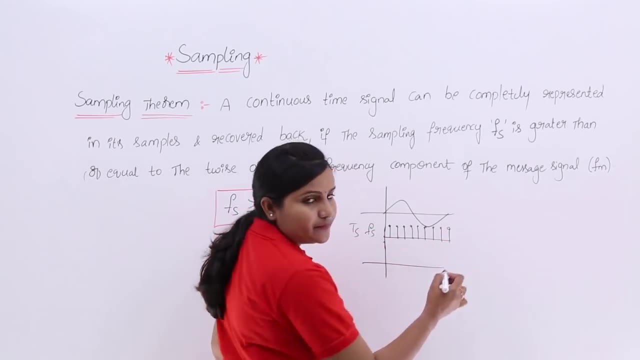 frequency fs. this is the pulse trying with a frequency fs. So that means time period, ts. ts is the time period between the samples. So by just multiplying these samples with this continuous signal you can convert the signal into its samples. So we can consider. 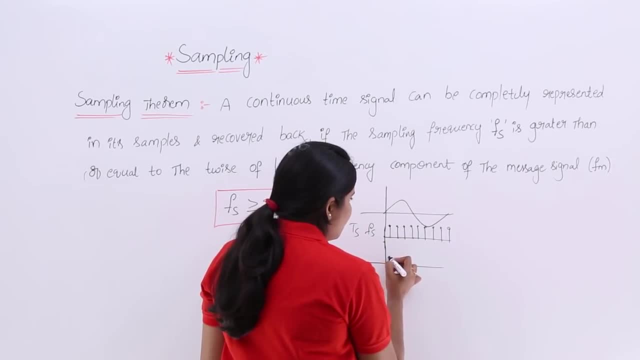 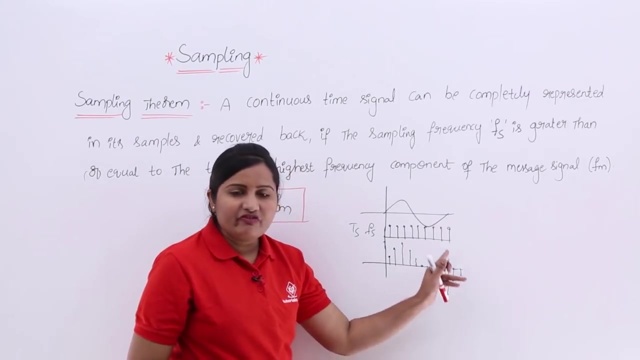 can completely represent your continuous signal into its samples, like this, like this: you can completely represent your signal into samples. So you are going to get this type of nature according to the samples you consider you are going to get this. So you are going to get the same signal shape which you are having in continuous form. that 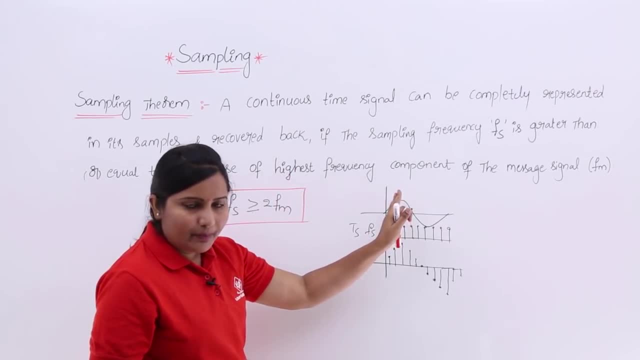 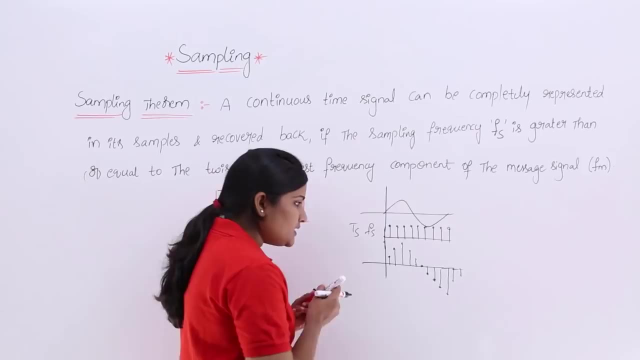 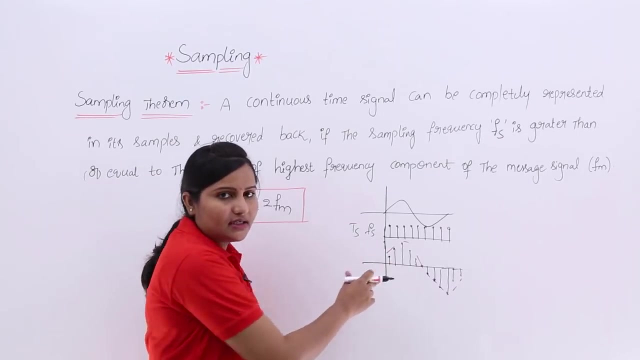 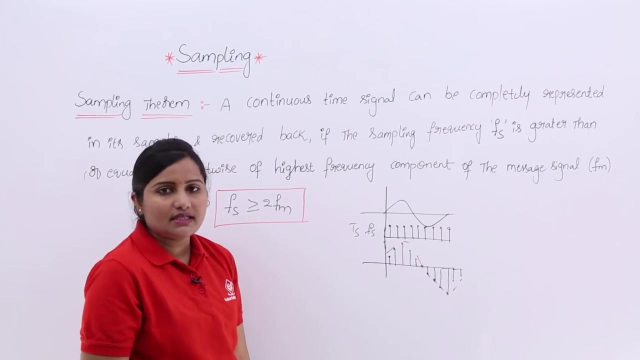 means a continuous signal. we can completely represented in its samples. If you want to reconstruct your continuous signal you can trace your signal here itself. you can see by this sampled signal. this is called as sampled signal. that means converted continuous signal. after conversion into discrete, that is called as sampled signal. This sampled signal is: 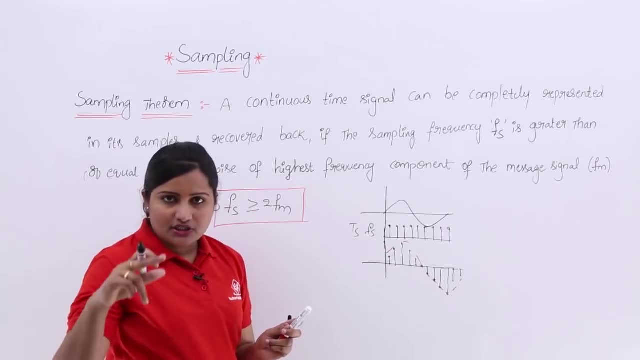 in the form of continuous. only that will take you to the continuous form. So this is the structure of continuous signal. So, and if it is in this form, then you can recover back your signal. if you want to recover back your signal, you just take the envelope. 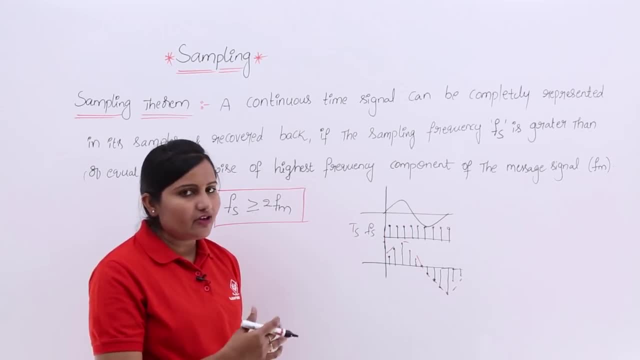 of this signal or you are having another process that I will show you in the next class how you will reconstruct your signal. So that means you need to consider transform of this sampled signal. after getting transform of this sampled signal, you will take a spectrum. 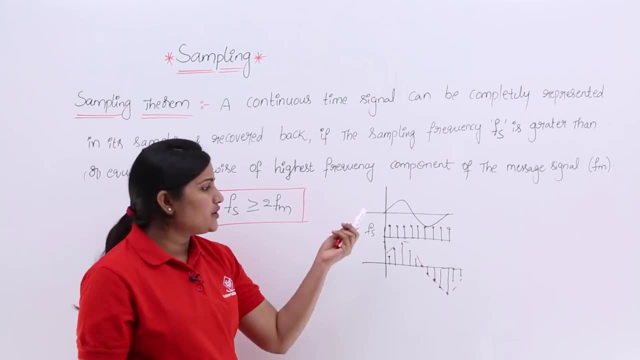 and you will take inversions. So this is the structure of continuous signal. So if it is in this form, then you can recover back your signal. So after some inverse transform you are going to get your signal, So that I will show you in the next class how you will get spectrum of this signal and how we 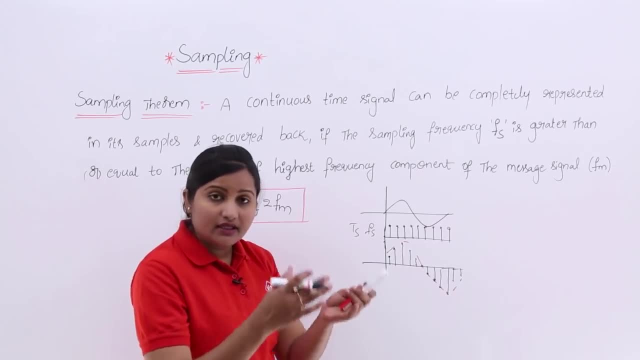 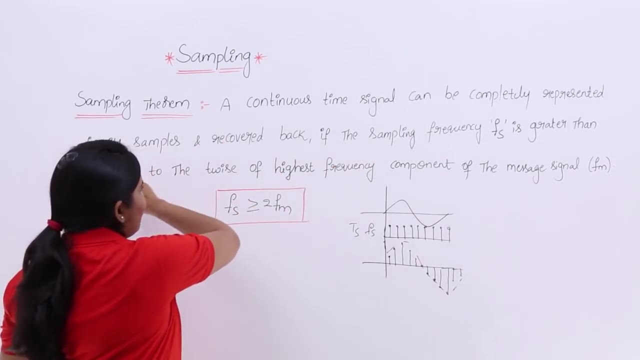 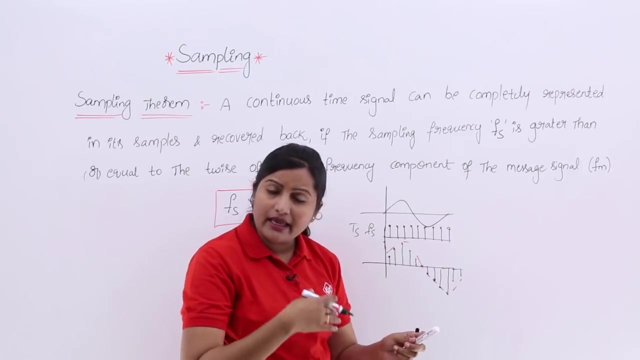 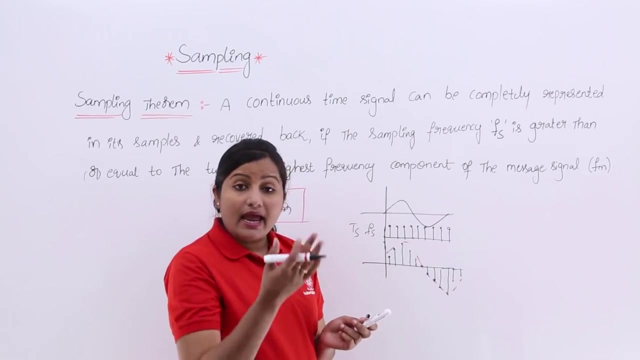 will reconstruct our message signal again in the derivation. I will show you So now in the statement I given you a continuous time signal can be completely represented into its samples. I am not, I am not converting partially, I, I can convert completely any continuous signal I can represent in its samples completely and can be recovered back also I can recover. 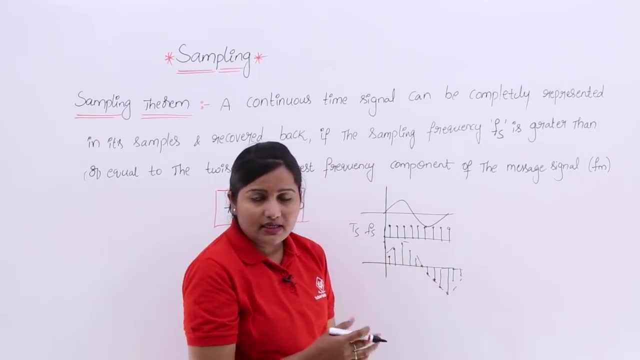 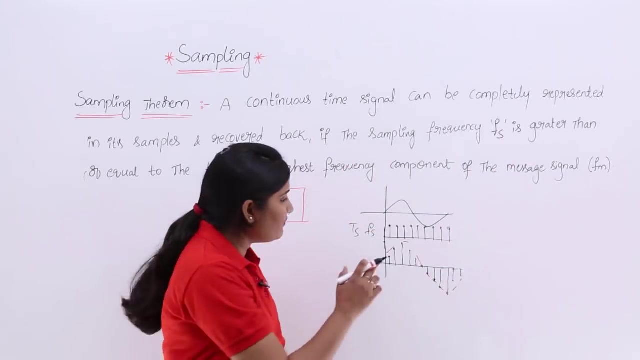 back this signal. If I am having this sampled signal, I can recover back my original continuous message signal whenever. but to do all this process- that means to completely represent to its samples and to recover back completely perfectly- we need to follow a condition. So if this is the condition, if the sampling frequency, sampling frequency is nothing but, 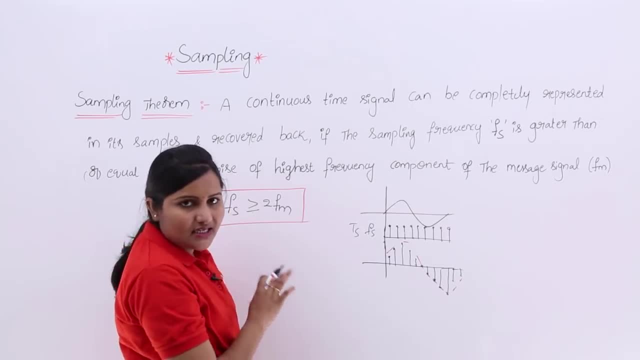 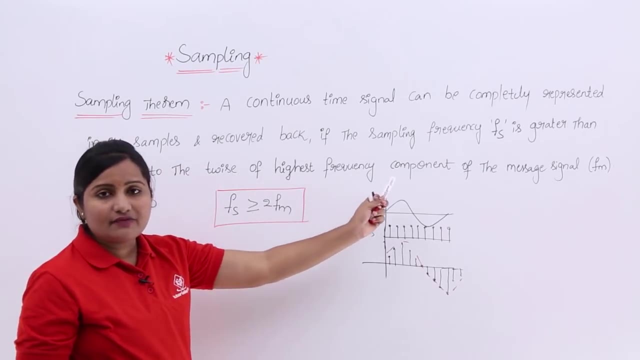 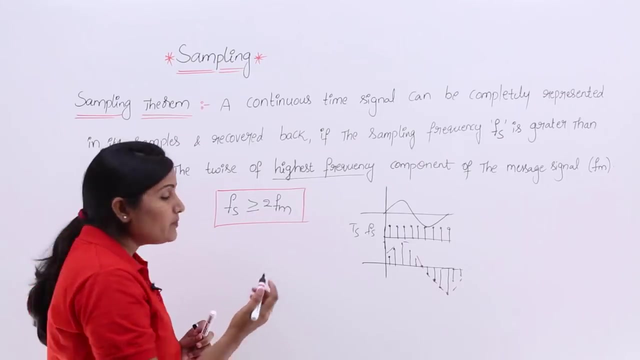 frequency of pulse train If sampling frequency fs is greater than or equivalent to twice the maximum frequency or highest frequency component of the message signal. I want to discuss with you about the highest frequency component of message signal. For example, if you are having any message signal like this, it is having two or three components. 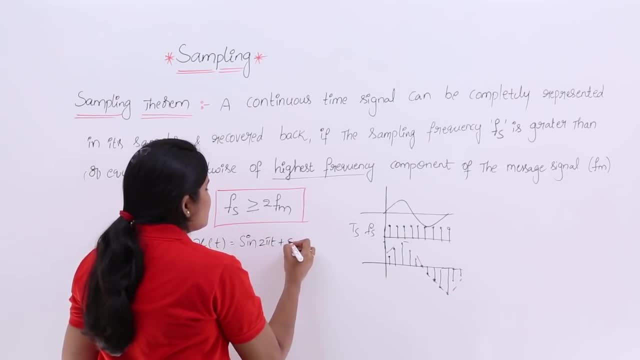 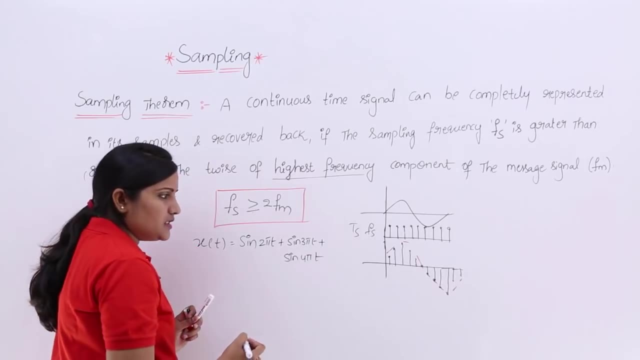 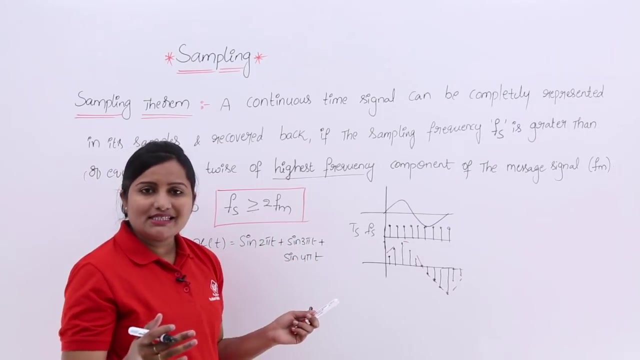 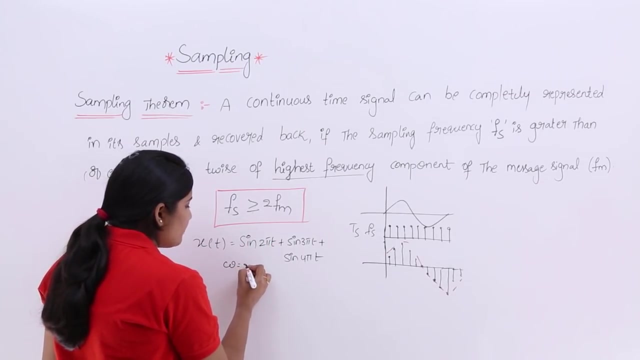 Sine 2 pi t plus sine 3 pi t plus sine 4 pi t. these are, these are your message signal components. by observing your message signal itself, you can say: your message signal is having three frequency components. That three frequency components are omega is equal into. 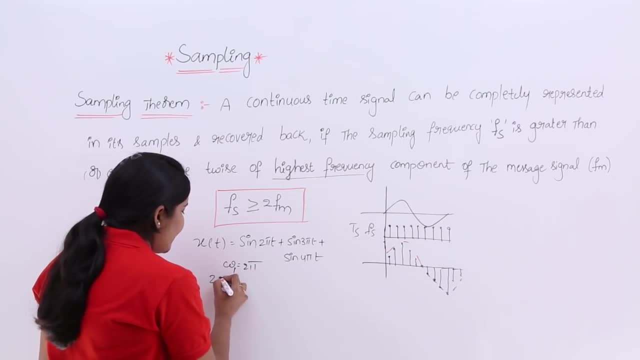 2 pi. So that means omega 1, I am considering. so 2 pi, f 1. is equivalent to 2 pi. So here your F 1 is equivalent to 1 if you cancel 2 pi with 2 pi. 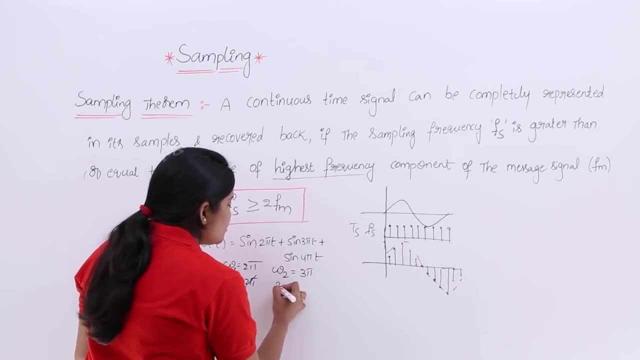 like that. omega 2 is equivalent to 3 pi 2 pi. F is equivalent to 3 pi. So pi pi- I am cancelling. F is equivalent to 3 by 2, 3 by 2 means 1.5.. So you can consider 1.5.. So now you are having. 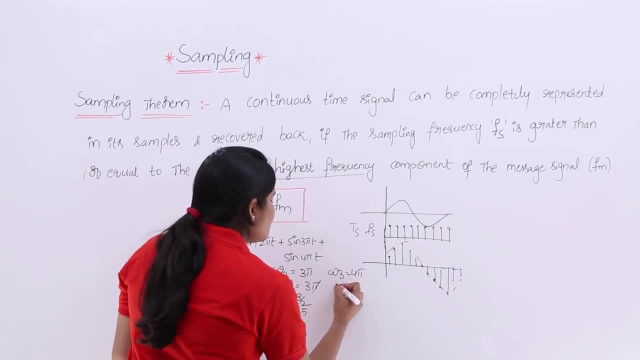 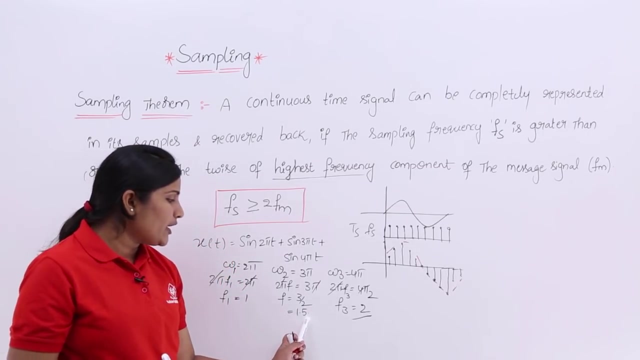 omega 3 is equivalent to 4 pi, 2 pi. F is equivalent to 4 pi. So 2 pi with 2 F 3 is equivalent to 2.. So you are having 3 frequency components. each of frequency 1 hits 1.5 hits and 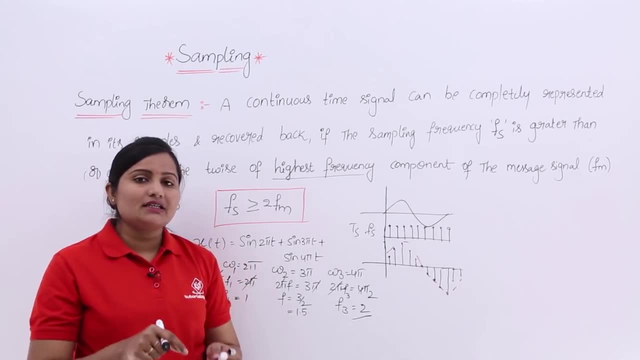 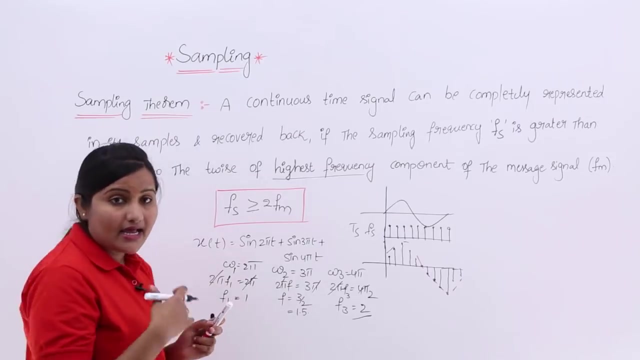 2 hits Now, which you can consider as frequency of your message signal. this is very important point: Which component you will consider as message frequency. So this is very important point: Which component you will consider as message. frequency means whatever highest frequency component is there that is considered as message. 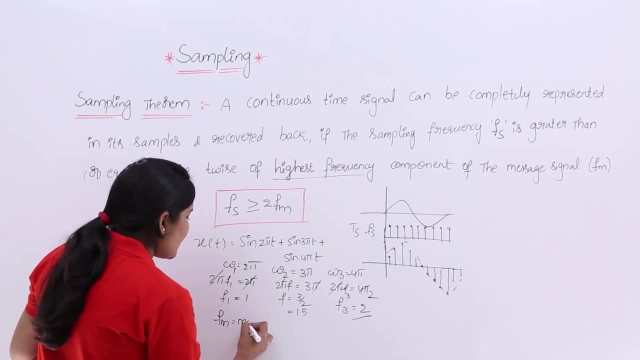 frequency component. That means f m is equivalent to maximum of f 1 comma, f 2 comma, f 3, this is f 2. So f 3.. So this is equivalent to maximum of 1 or 1.5. 2 means 2 can be considered. 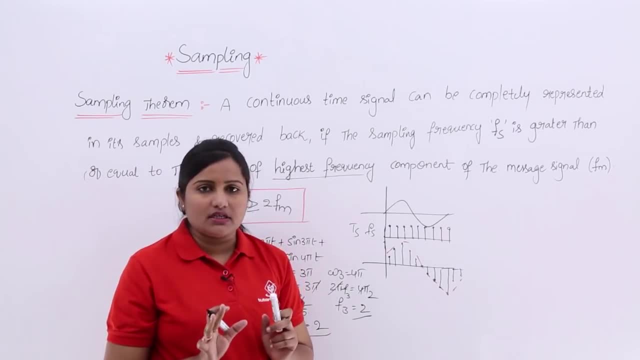 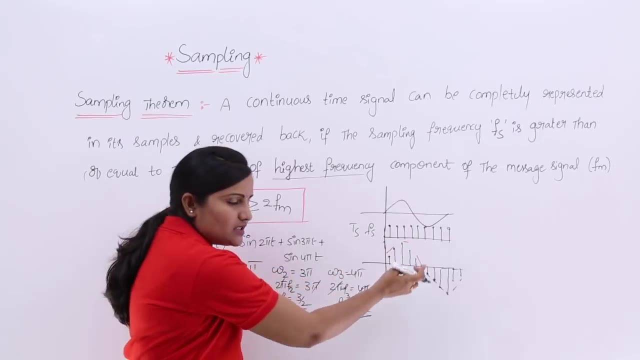 as your f? m. So like this way you need to consider So as this as a basic case. So in the statement they given, to construct completely, to represent into its samples any continuous signal. If you want to represent in its samples completely and to recover back your sampling. 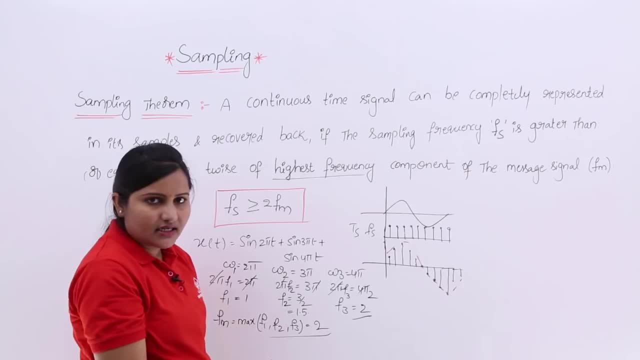 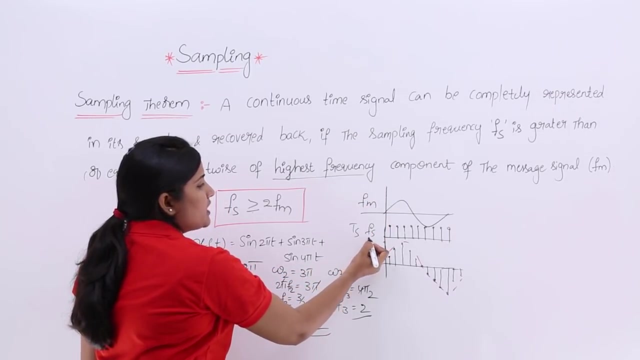 frequency, whatever sampling train. here you are considering that sampling frequency must be greater than Are equivalent to your twice the maximum frequency component of your message signal. So this f? m is the message frequency So you need to consider. So this f? s at least equivalent. 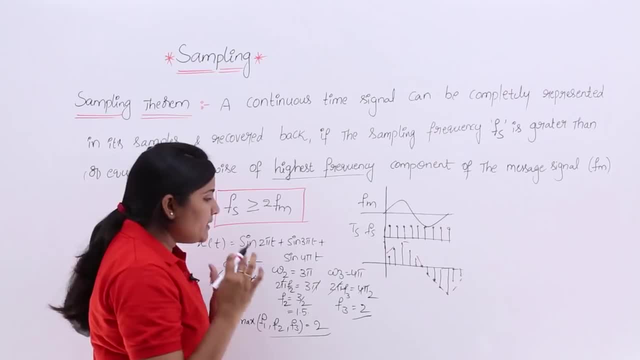 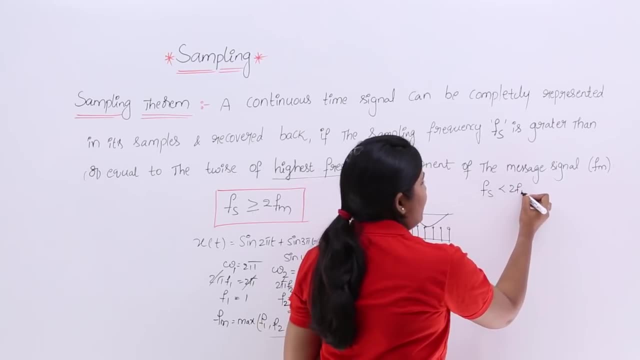 to twice this f m. So that means, for example, what will happen if you violated this condition? that means f s less than 2 f m. if you consider like that, Actually, you need to consider f s greater than or equal to 2.. 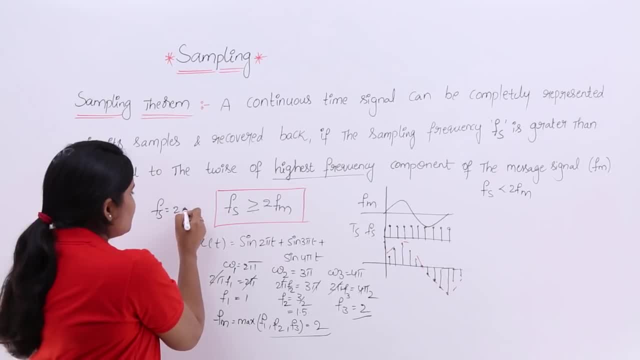 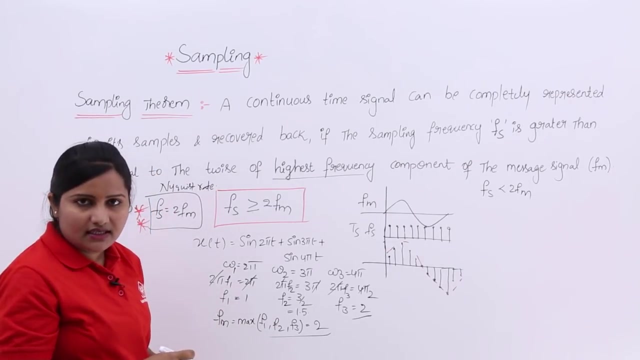 f m in this least condition is f s is equivalent to 2 f m. this is called as Nyquist rate. Nyquist rate. this is called as Nyquist rate. this is also very, very important. why? because in so many exams they are asking: what is the Nyquist rate of the signal if message frequency is? 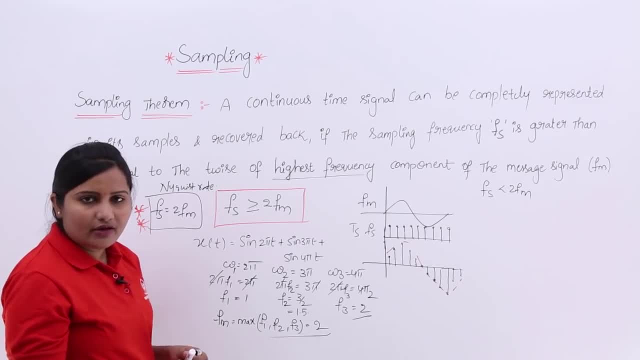 this: if highest frequency component value is 2 hedges, what may be? the Nyquist rate of your signal is equivalent to 2 f m, So this is equivalent to 4 hedges. maybe Nyquist rate of your signal that means at least 4 hedges. 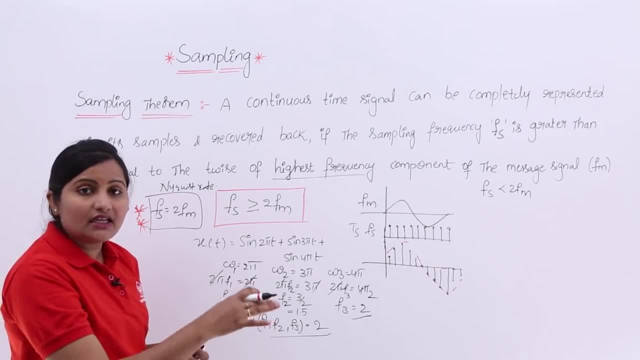 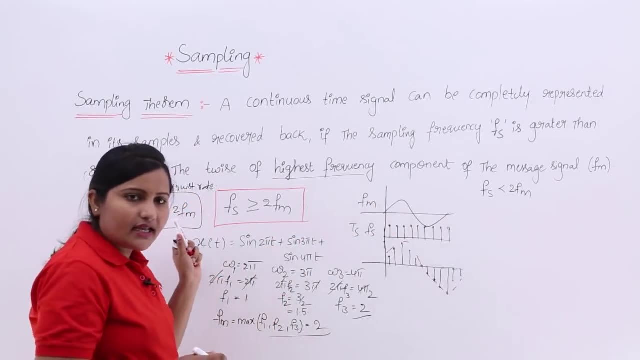 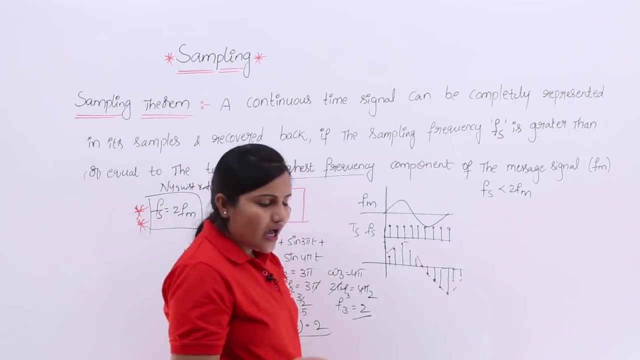 you need to consider to convert a 2 hedge signal into its discrete form. So that is the meaning. So here, this is the Nyquist rate. if you violated this Nyquist and sampling rate- sampling theorem, that means if f s less than 2, f m generally- what will happens? I want 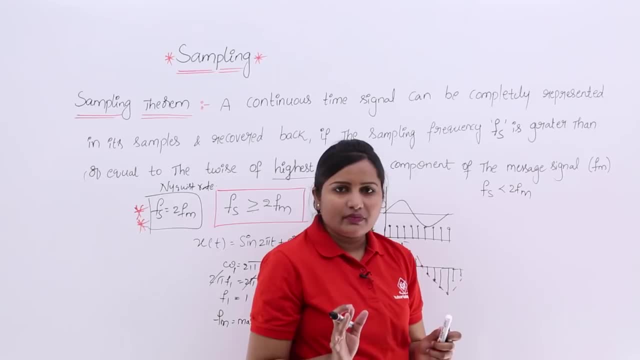 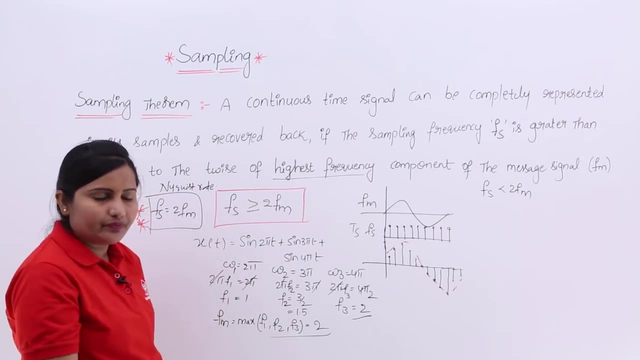 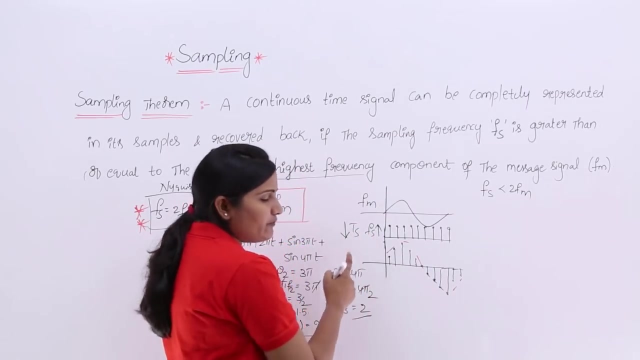 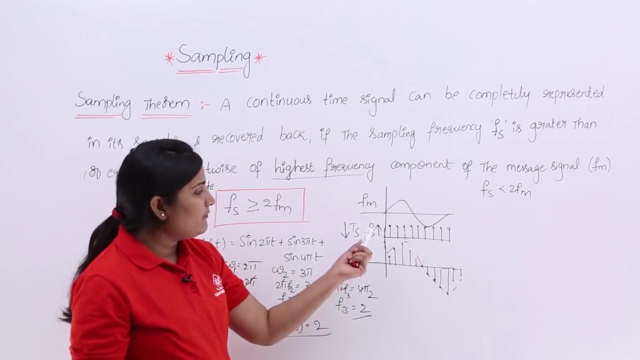 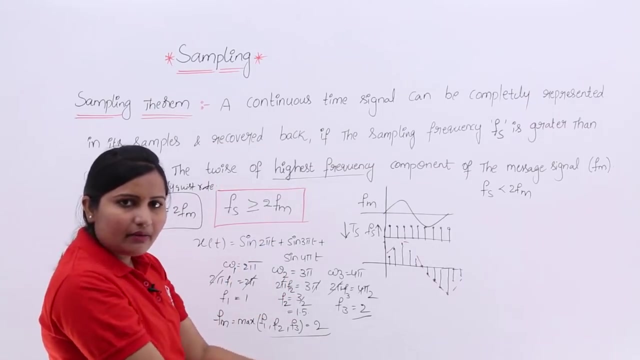 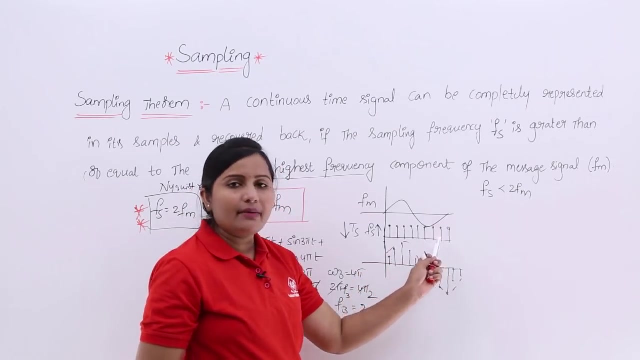 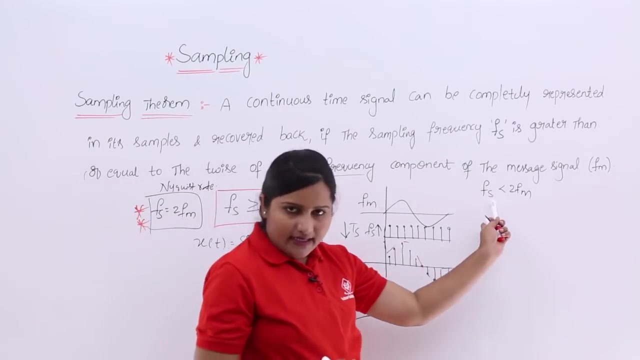 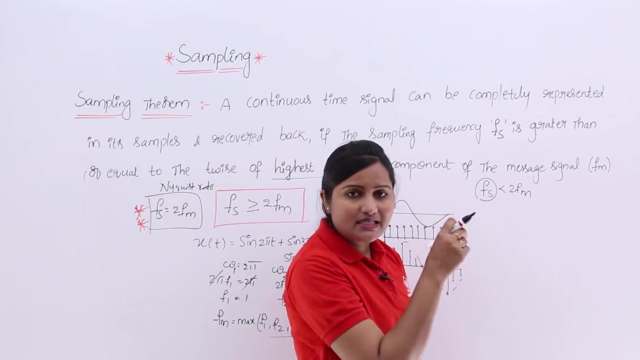 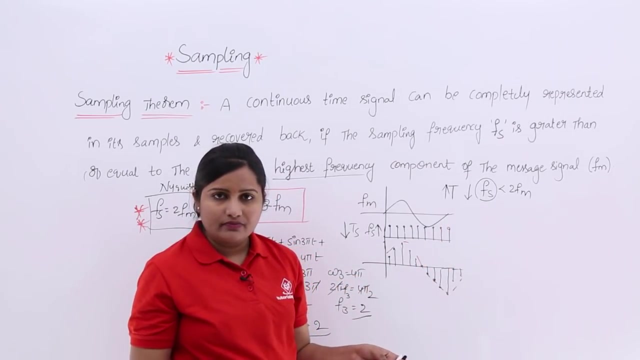 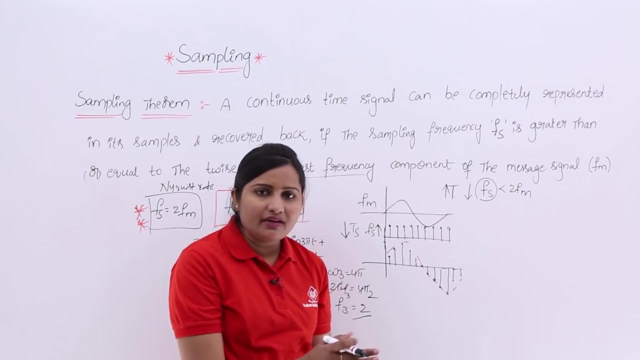 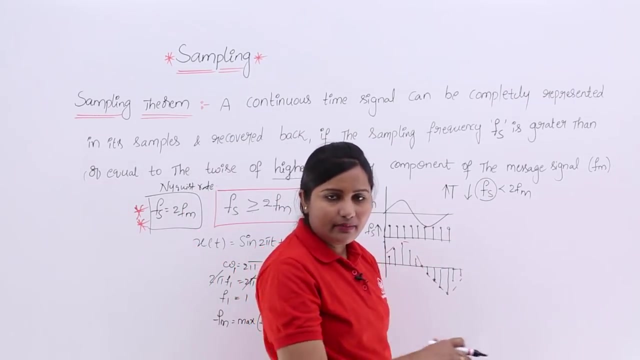 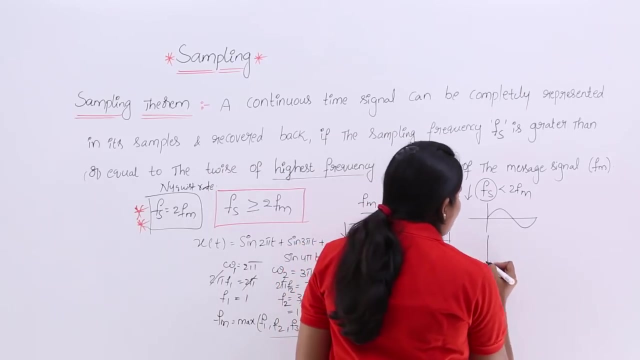 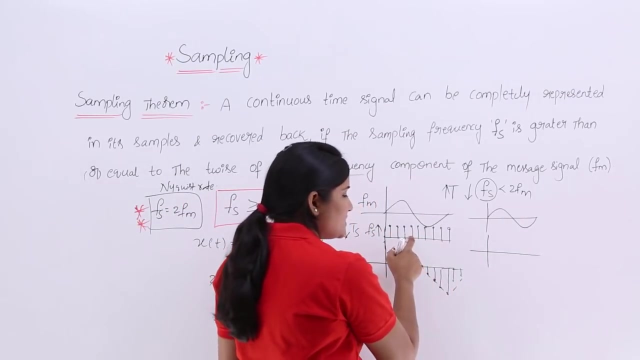 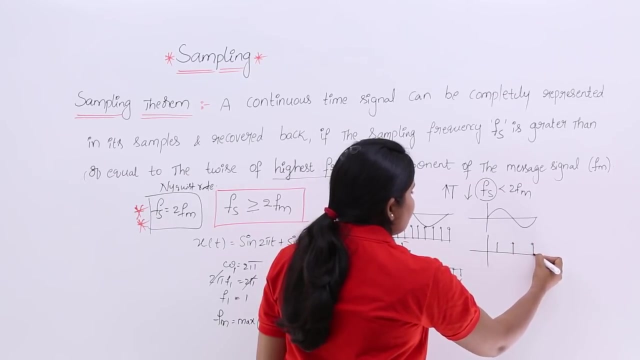 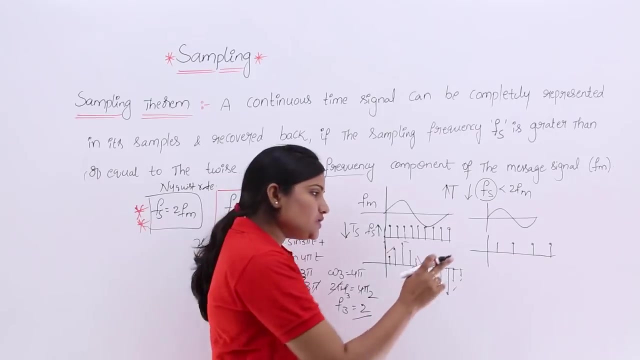 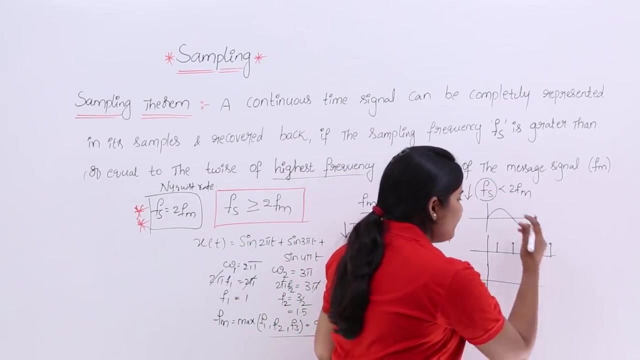 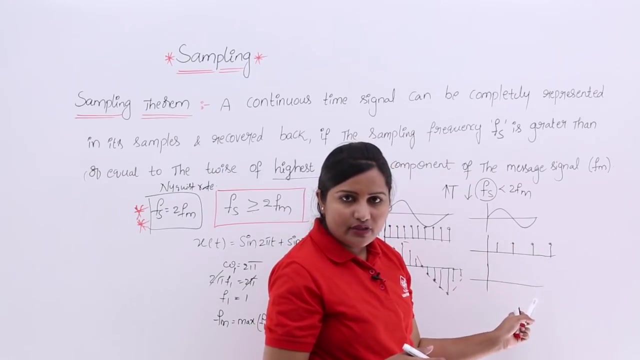 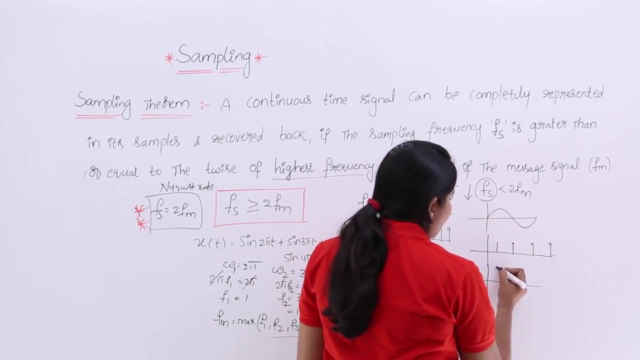 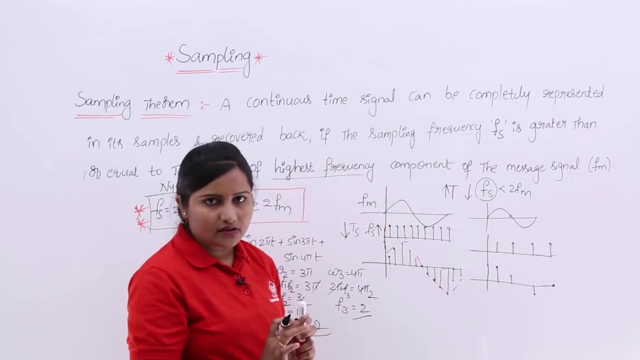 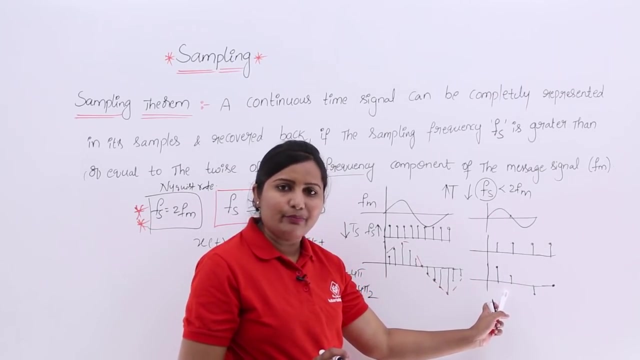 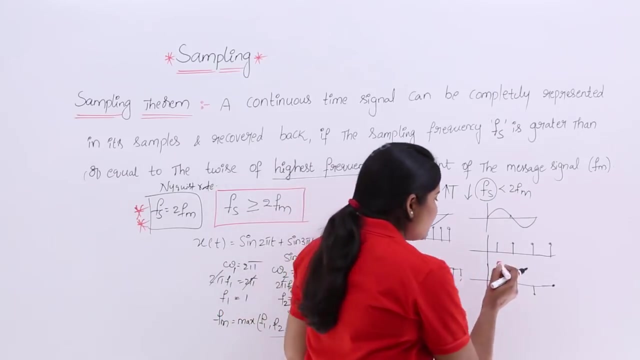 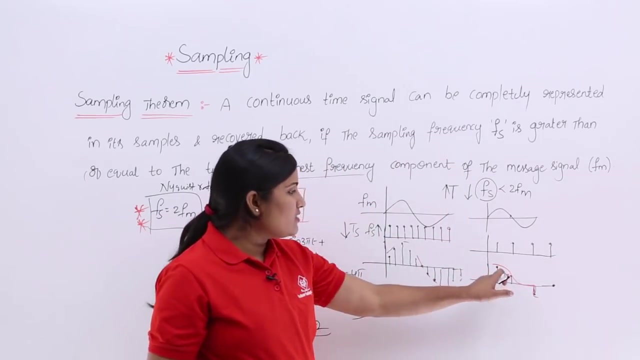 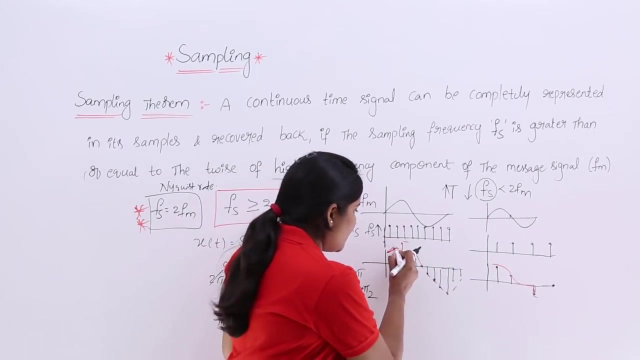 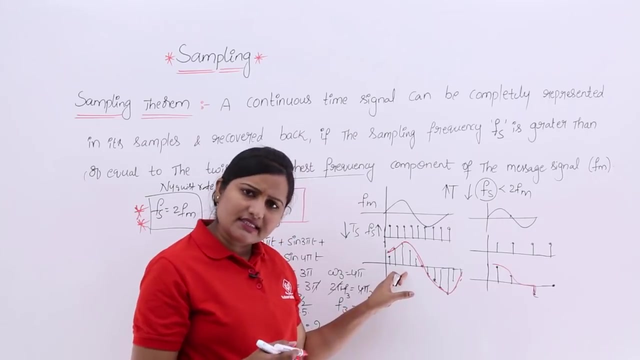 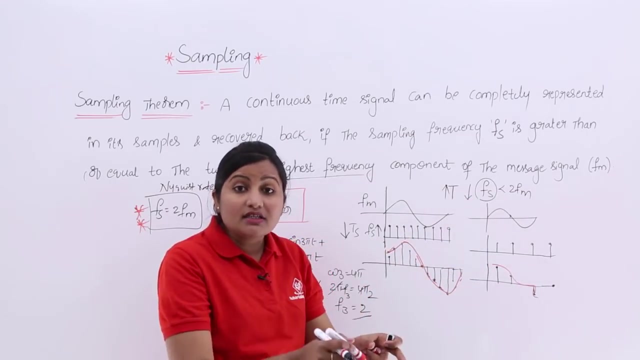 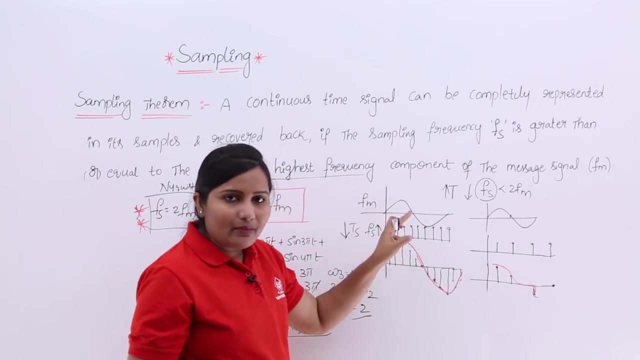 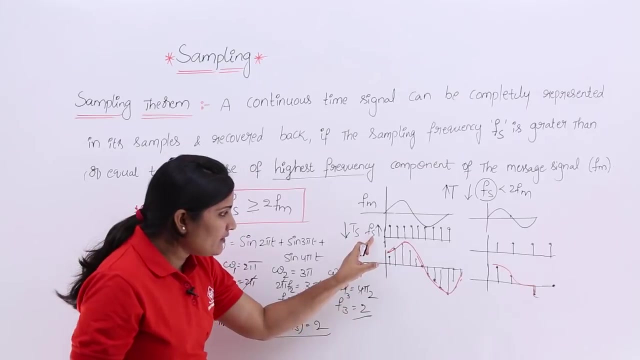 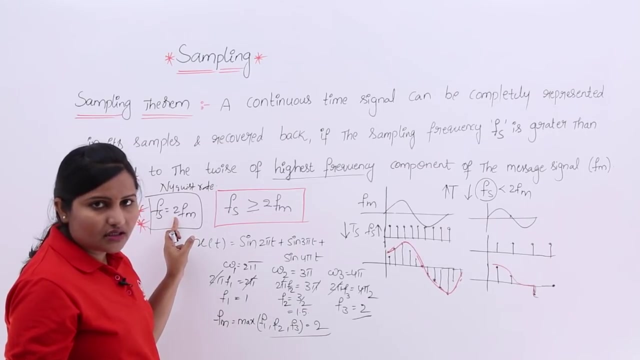 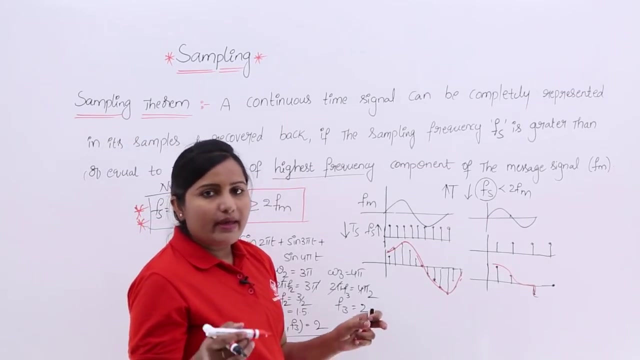 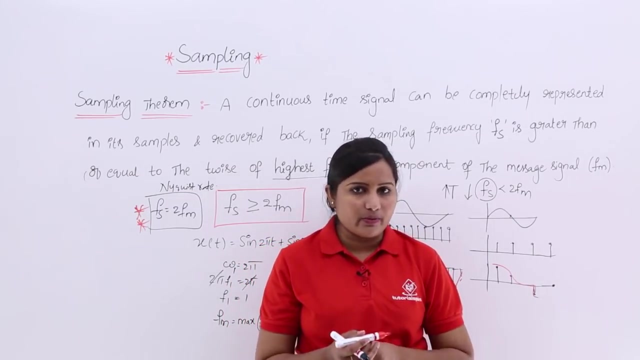 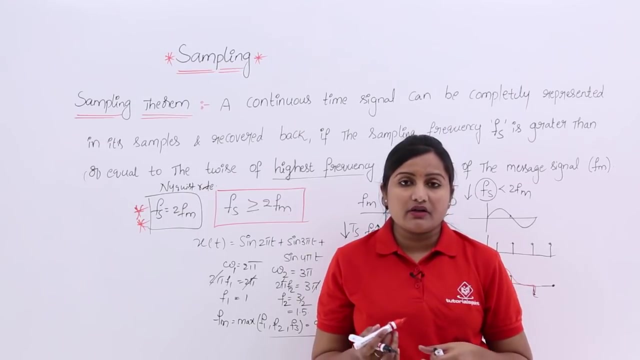 to discuss with you the general case, practical case. So this is the maximum of all that frequency components. So this is about sampling theorem. in the next class we are going to get the proof for sampling theorem. that means we are going to verify the sampling theorem in the next class itself.